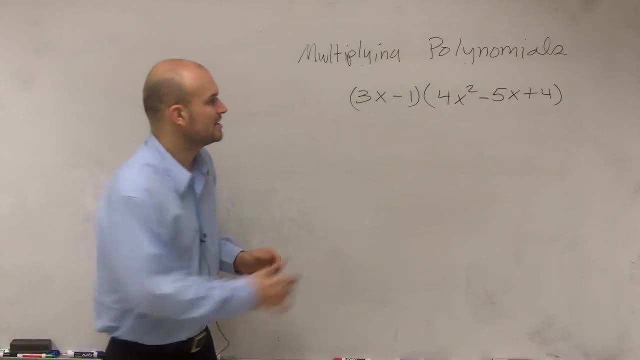 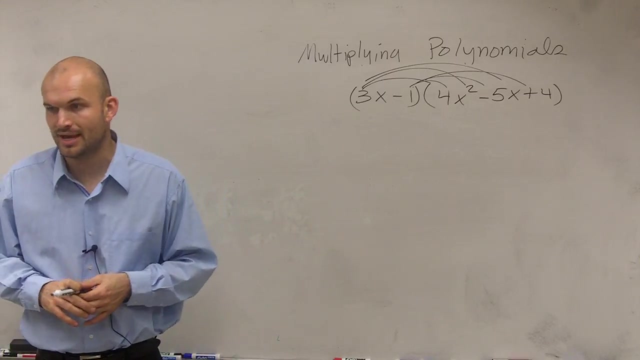 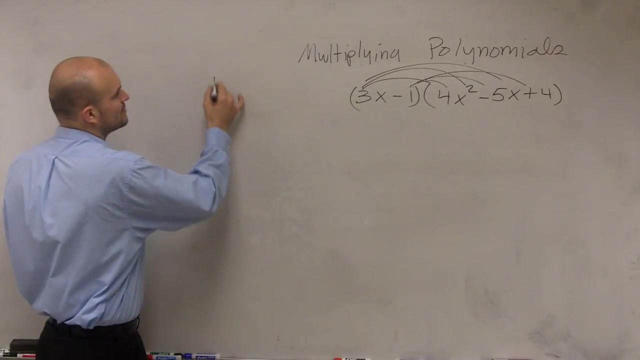 you with a way to easily organize this information, Because in reality, you have to multiply this term times every term, and then you have to multiply this term times every term, And guess what? It's a great way to get confused and make a mistake. So what I want to do is I want to give you a tool that you can use when multiplying any type of polynomials to each other. So what we need to remember is the good old rectangle: If I said this is 4 and this is 2,. 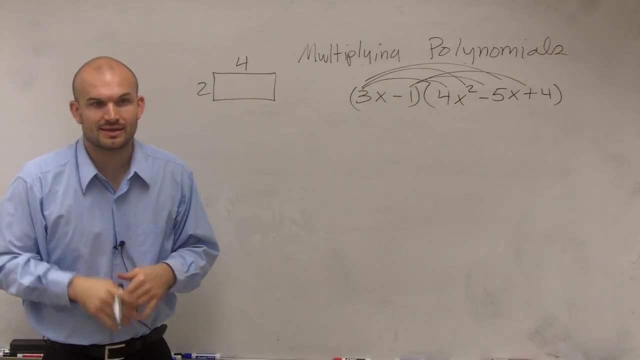 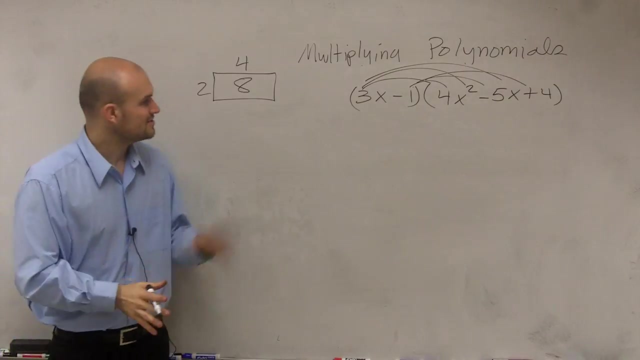 right. When you multiply them, you're going to get the what Area right. So you multiply them, you get the area. Now, one thing I want you guys to notice is what if I broke it up, If I broke this box, if I said this was 2, and I broke that up into two sections and then I broke this up into 4,, right Where this is 1 plus 1 plus 1 plus 1,. 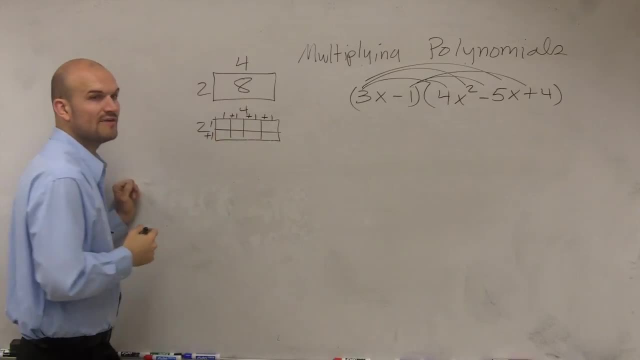 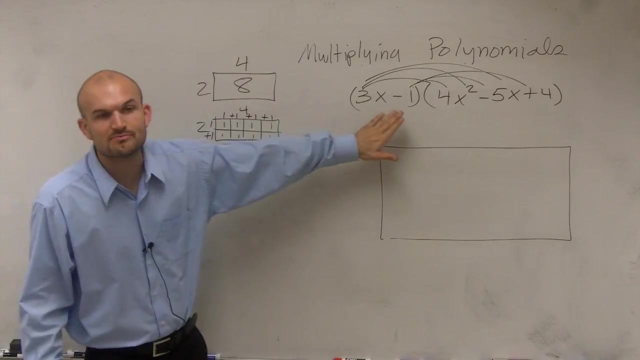 and this is 1 plus 1.. Now, if I found the area of each one of these little boxes, let's see if it adds up to 8.. Right, 1 times 1 is 1.. 1 times 1 is 1.. Does all these little boxes add up to 8? Yeah, So we can break up a box. So what I'm going to do is I'm going to create a rectangle And, rather than using these easy numbers, I'm going to use my polynomials. So here I have two of them, right? So I'm going to say I have two. 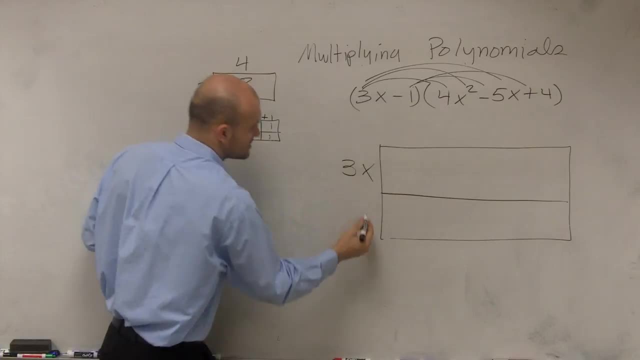 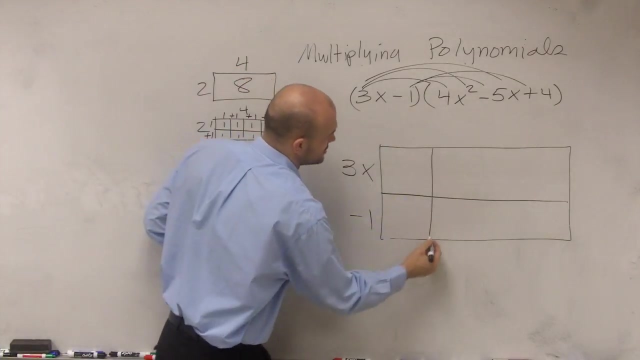 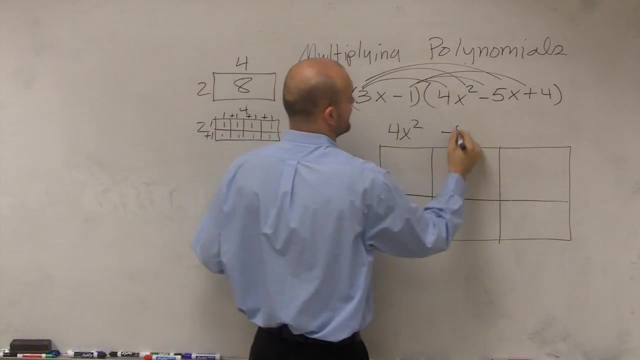 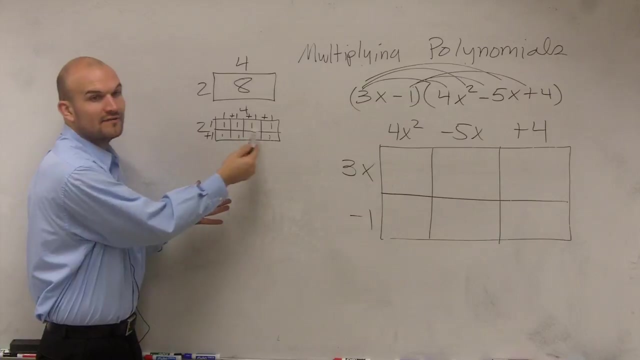 monomials. So I'm going to say the first one is 3x and the last one is negative 1. Then over here I have 3.. So I'm going to break up my box into three different sections. So the first term is 4x squared, Next one is negative, 5x and the last one is 4.. So now, like I did before, I'm just going to find the area of every single box and then add them up together, So 3x times 4x squared.